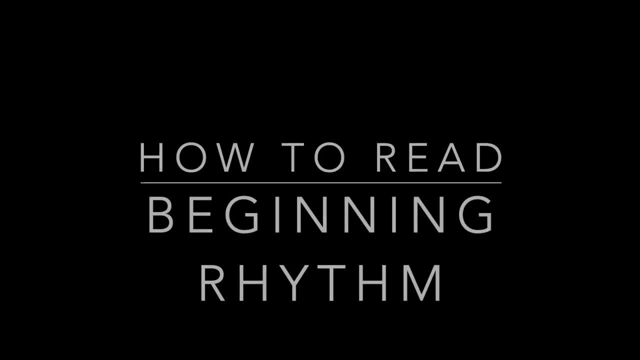 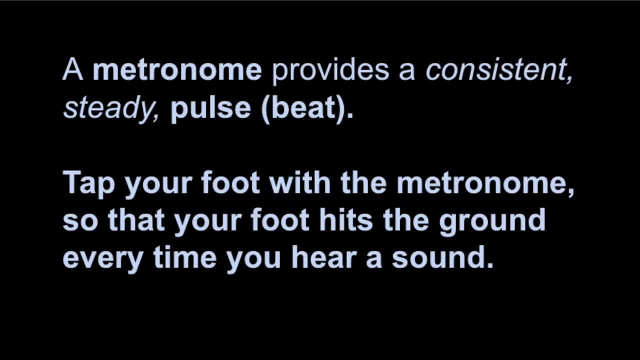 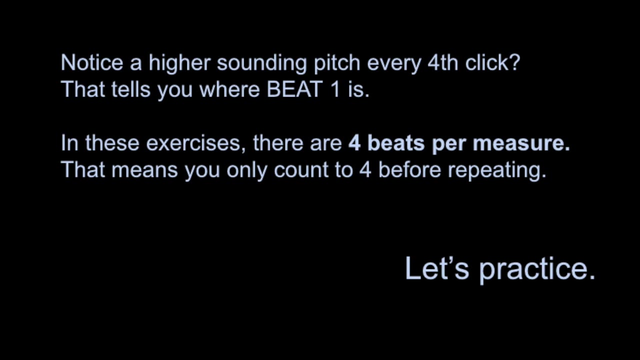 In this exercise we're going to practice beginning rhythm. This is a metronome. A metronome provides a consistent, steady pulse or beat. Tap your foot with the metronome so that your foot hits the ground every time you hear a sound. Do you notice a higher sounding pitch? every fourth click? That tells you where beat one is. In these exercises there are four beats per measure, which means you only count one, two, three, four. before repeating, Let's practice. 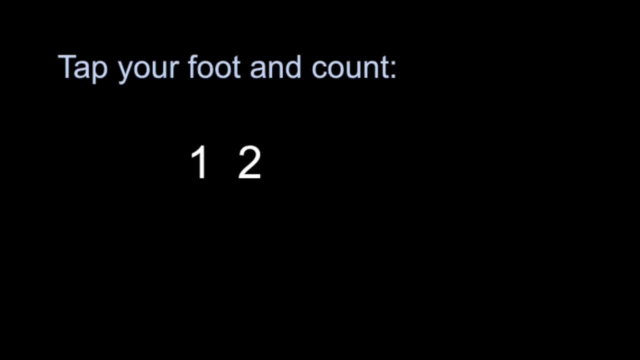 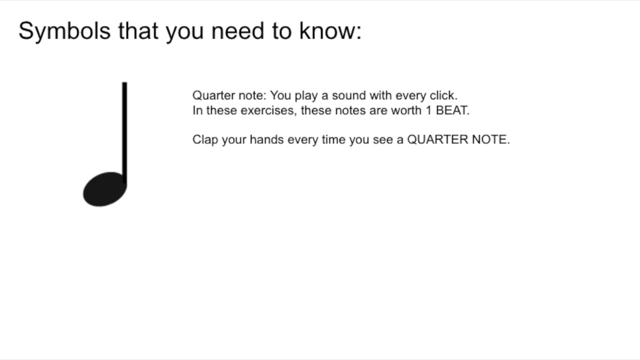 Ready go One, two, three, four. Repeat One, two, three, four. Great. Were you counting out loud and tapping your foot? If not, go back and try that exercise again. Let's move on. This is a quarter note. In our exercises, a quarter note equals one beat In addition to tapping your foot and counting out loud. now you have to clap your hands every time you see a quarter note. 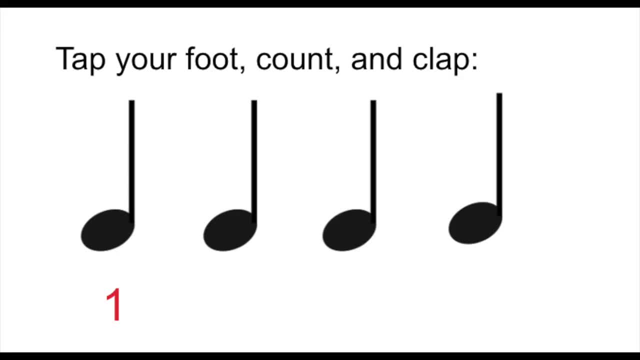 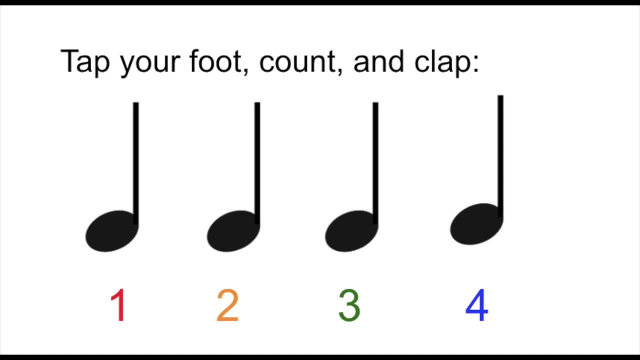 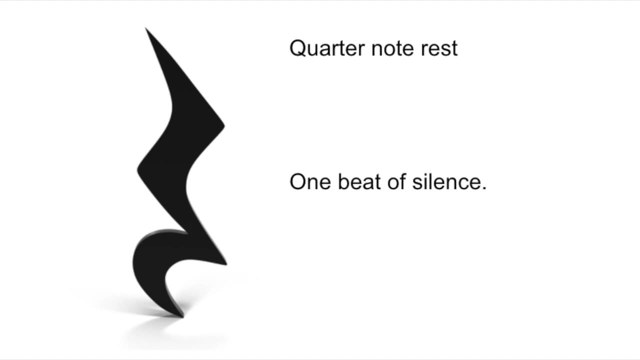 Let's practice Ready go: One, two, three, four. Repeat: One, two, three, four. Sometimes you'll see this symbol, which is a quarter note rest. It's the opposite of a quarter note. Instead of one beat of sound, you're going to have one beat of silence. 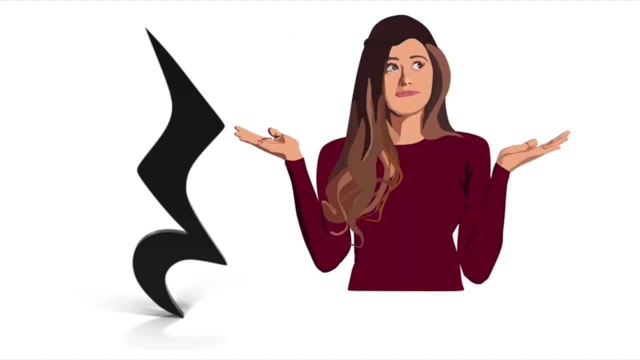 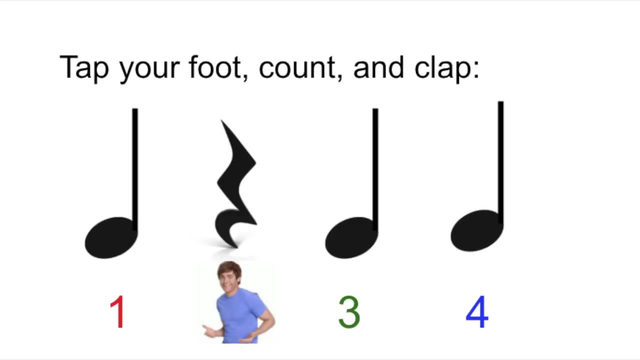 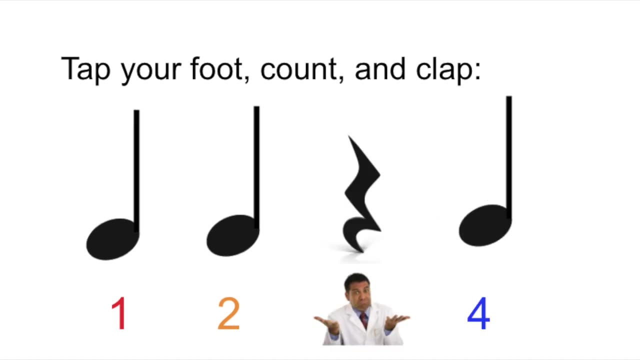 To practice this. instead of clapping your hands together, hold your hands apart to show that you understand that this is a rest. Let's practice a few of these Ready go: One, two, three, four: 1, 2, 3, 4, 1, 2, 3, 4, 1, 2, 3, 4,. last one: 1, 2, 3, 4.. 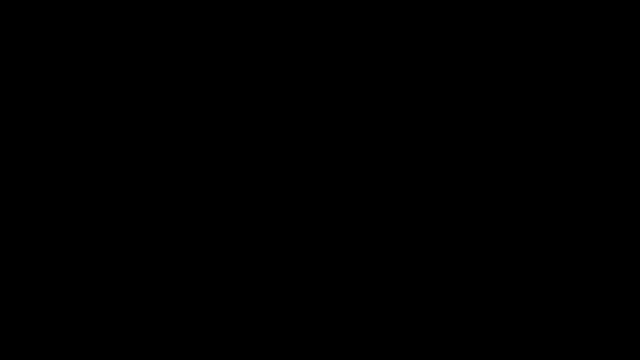 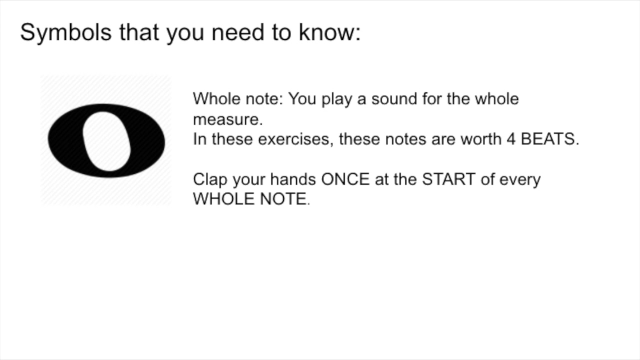 If you understand how to play quarter notes and quarter note rests, it's time to move on to a whole note. This might be review or it might seem easy, but it's really important that you have a solid understanding of these fundamental rhythms so that we can move on to more advanced exercises. 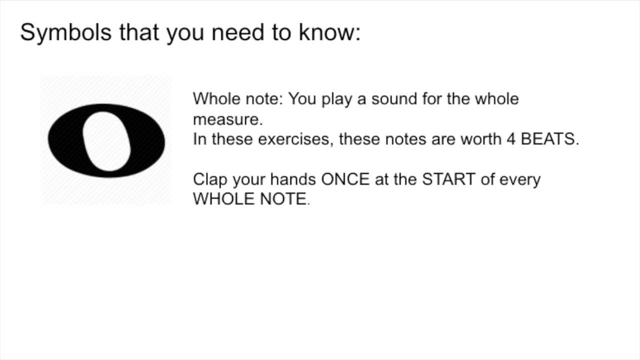 This is what a whole note looks like. A whole note means you play a sound for the whole measure. In these exercises that we are doing, the whole notes are worth four beats. You clap your hands once at the start of every whole note and then you hold them together to indicate that you know that you are holding out the sound.